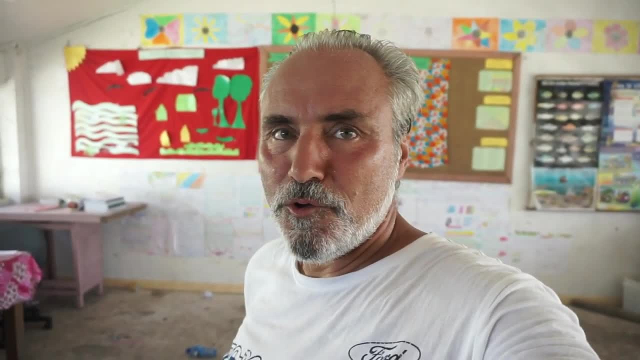 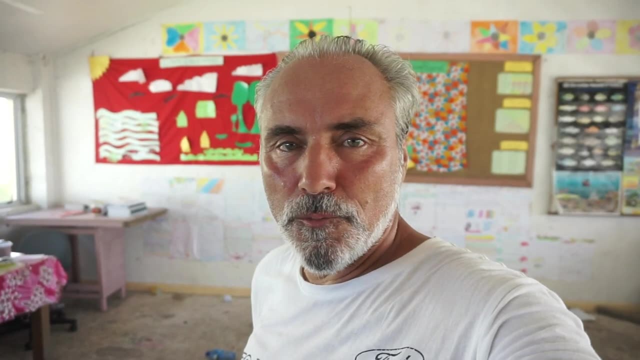 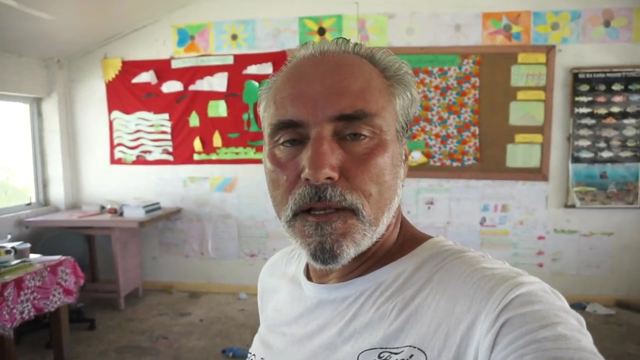 Hello, this is Vic. Welcome to my channel and thank you for viewing my videos. Today I'm in a beautiful, exotic and faraway country of Tuvalu. You may be asking yourselves now: where in the world is Tuvalu? Well, it is located about three hours north from Suva by plane. 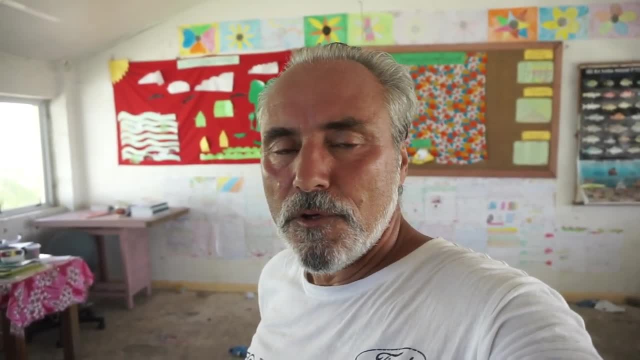 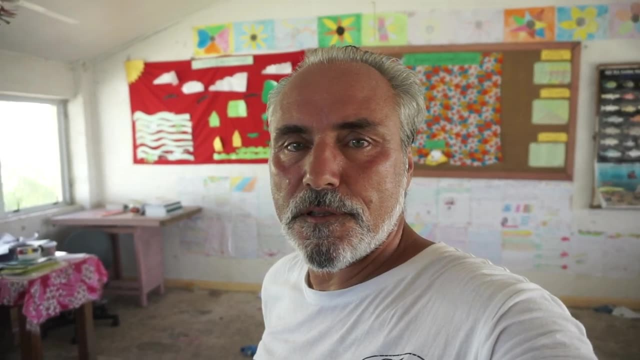 And Suva is the capital of Fiji. You can only get here twice a week by flight from Fiji, and that's about it. It is one of the most remote democracies in the world and it is a country of about 12,000 people. 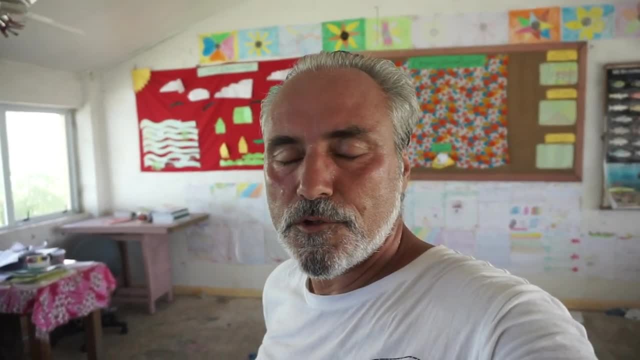 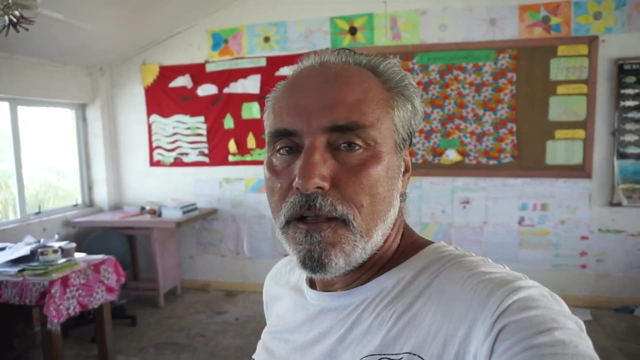 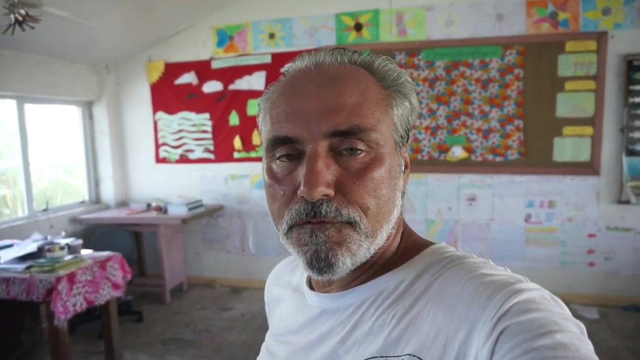 And it is one of the most beautiful countries in the world. So look at my channel for other videos so you can see what it looks like here in Tuvalu. In this particular video we're going to go in the Nauti Primary School, the big primary school here at Funafuti, the capital of Tuvalu. 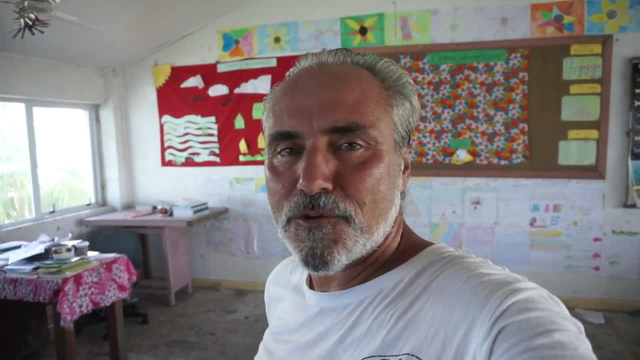 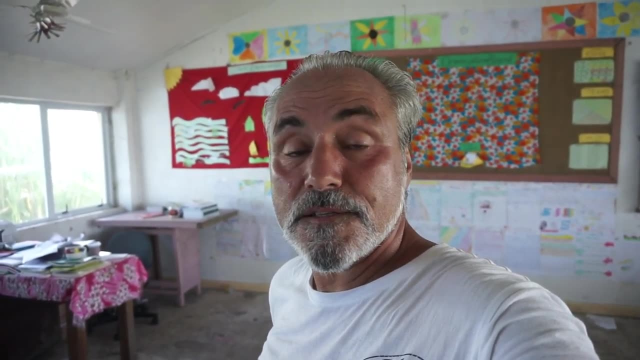 We're going to go inside the classrooms, Not that the school is in recession. We're going to see what the classrooms look like. So join me for the very, very interesting documentary. Here's the Nauti Primary School in Funafuti, the capital of Tuvalu in the Central Pacific. 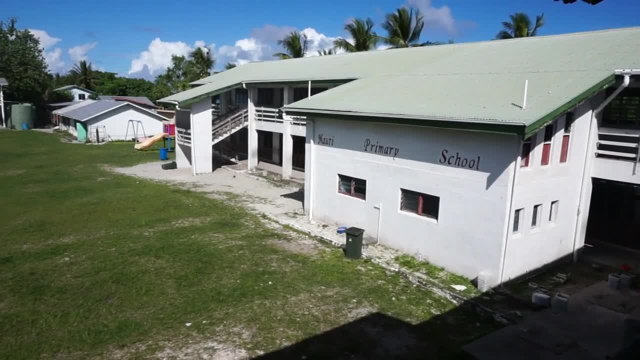 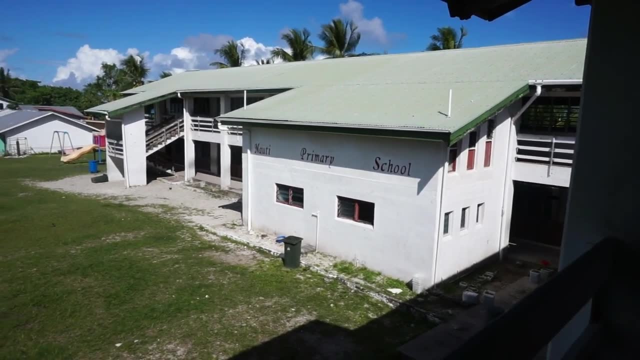 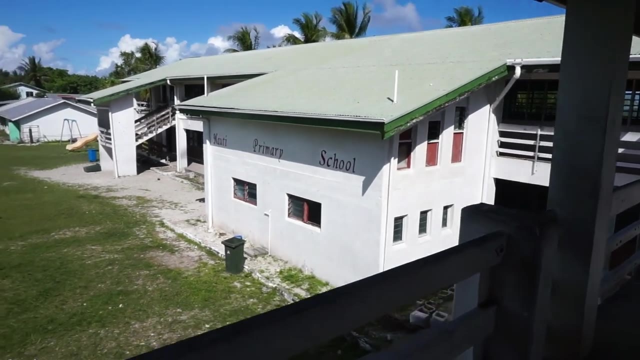 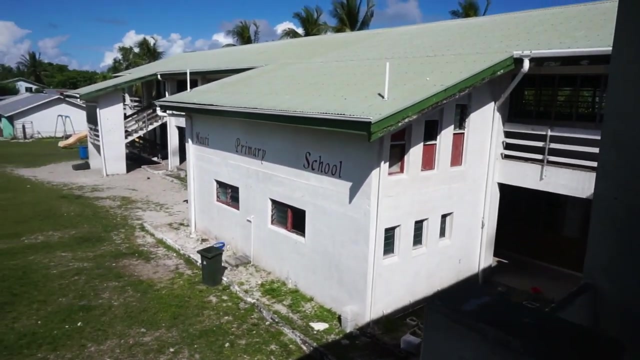 Wow, Let's go. And here is a view of Nauti Primary School From the second floor, where I am right now. Now, this is the school for grades 1 through 12.. Through 8. We're going to get a chance now to go inside some of the classrooms. 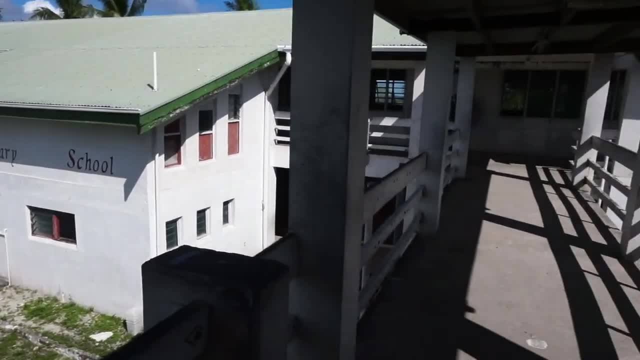 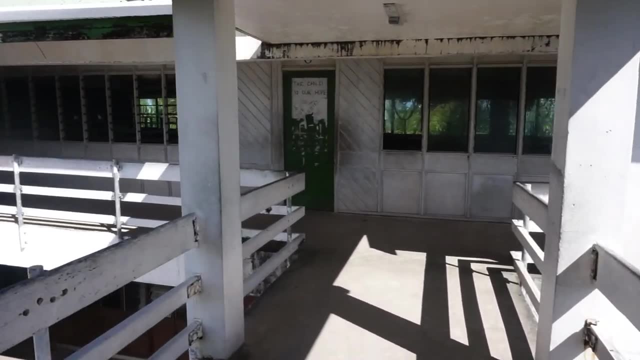 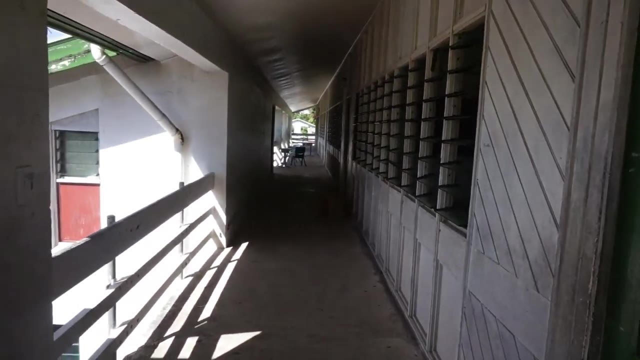 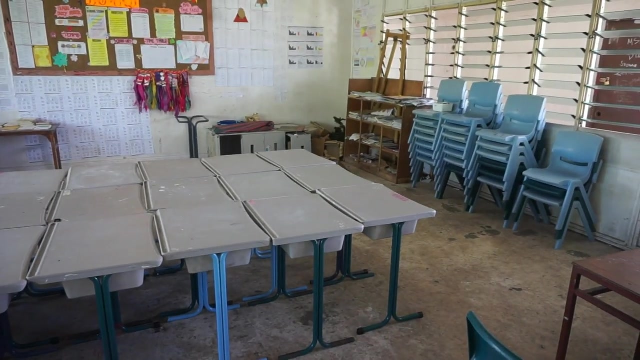 And videotape them. So you have never seen a classroom in a school in Tuvalu. Well, here's your chance. Let's get a view of the classrooms first, right there, Let's go in a couple of them. The school is in recession right now. 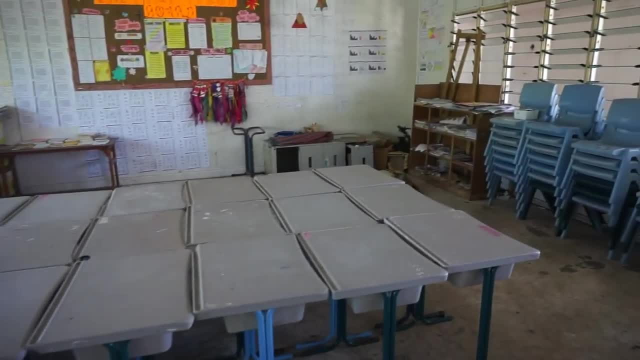 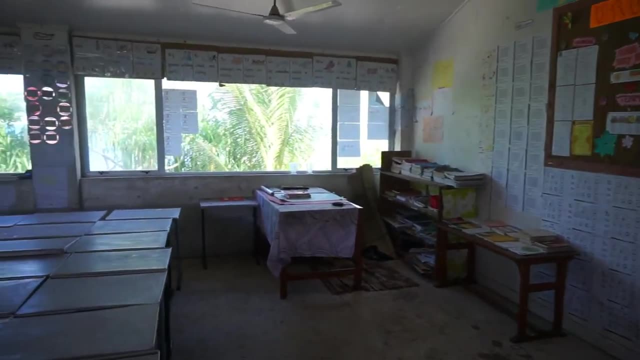 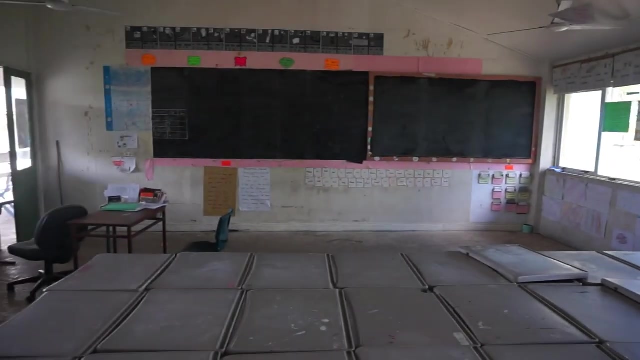 So there are no classes, But let's walk around. This is one of the classrooms here. Now, the windows here face towards the lagoon of Tuvalu, The famous lagoon, The beautiful lagoon. That's the board right there And these are the individual desks. 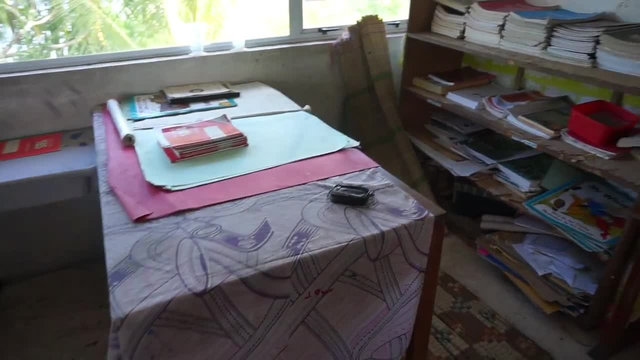 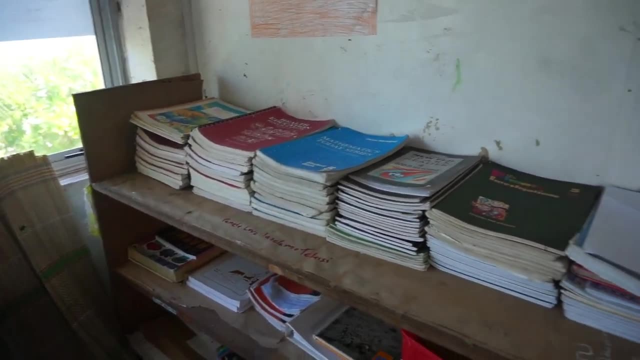 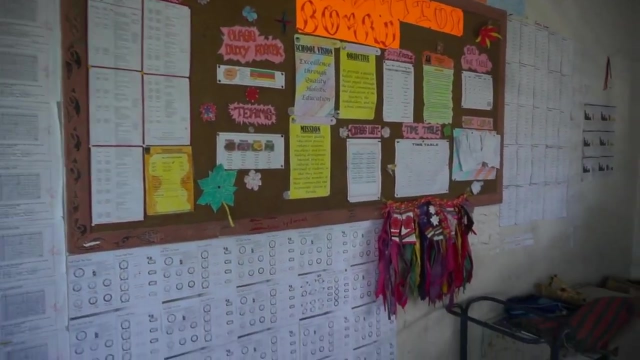 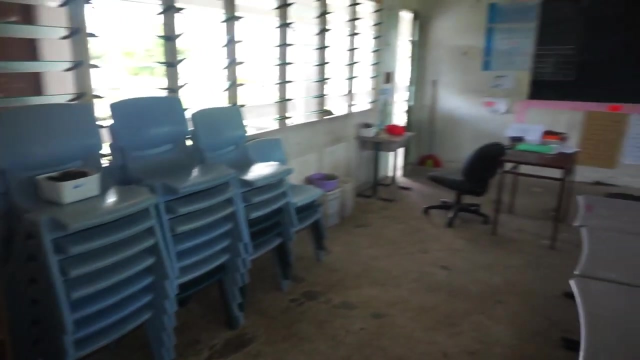 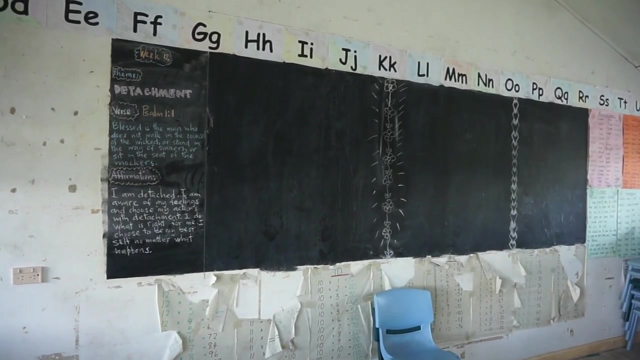 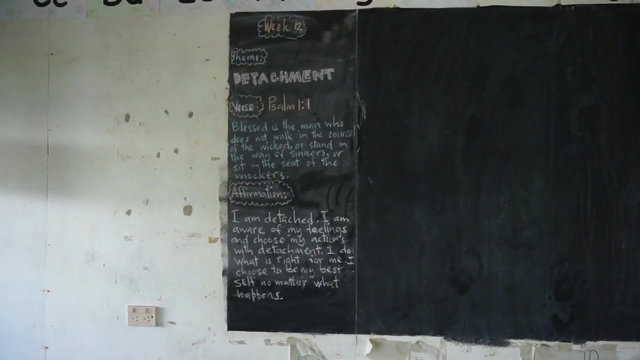 The teacher's desk. These are all the books I would imagine. Look at this. These are the chairs. Okay, I am inside a different classroom. Let's see here what the last class was about. This was week 12. And the theme was detachment. 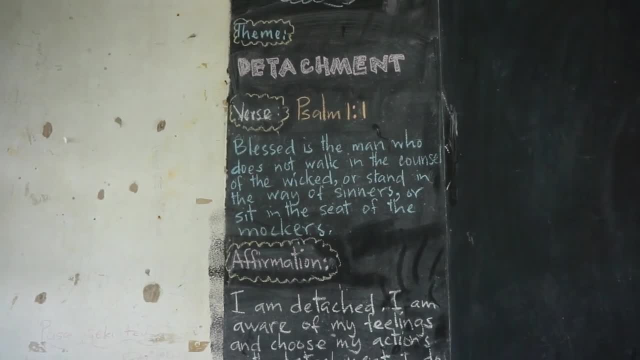 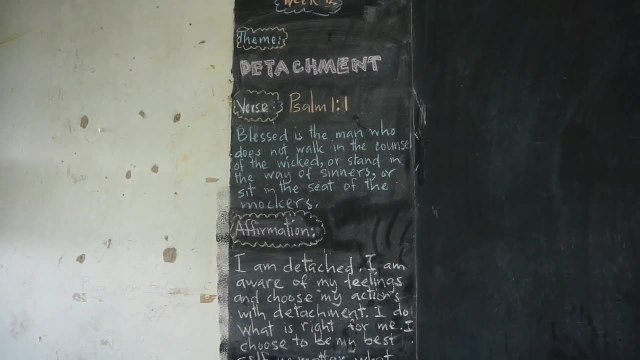 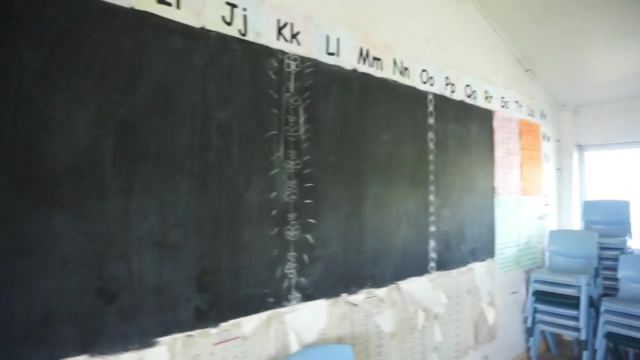 And it says here: Blessed is the man who does not walk in the counsel of the wicked or stand in the way of sinners or sit in the seat of mockers. You can see here Now: what's really important here is that. 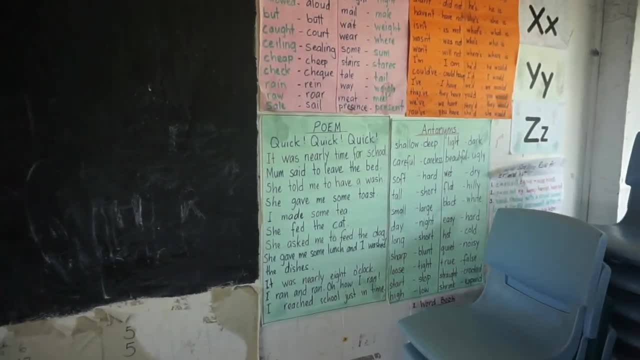 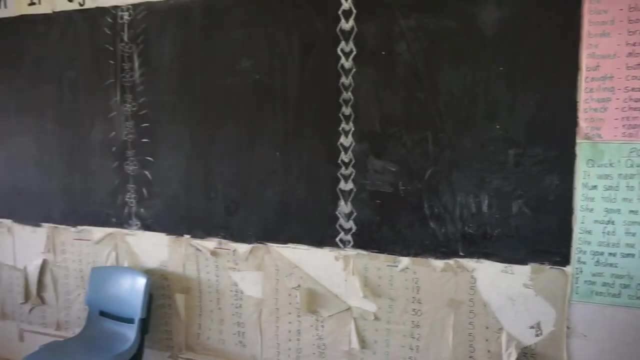 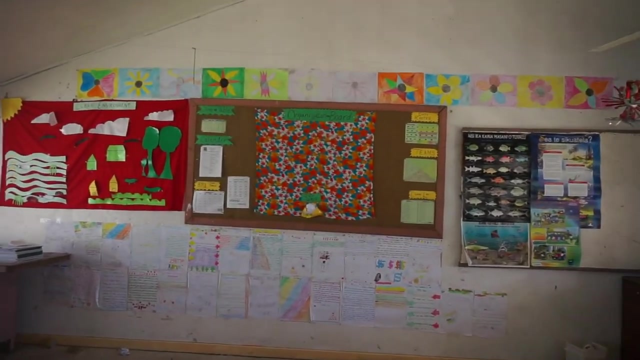 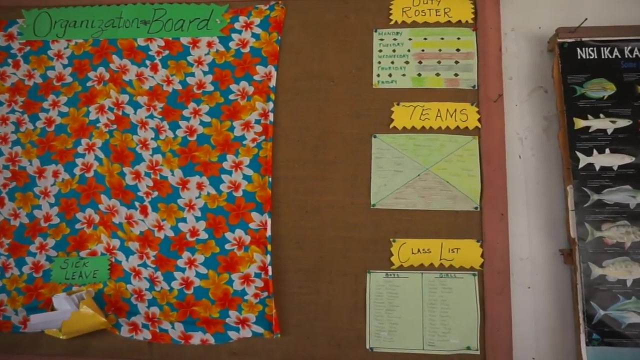 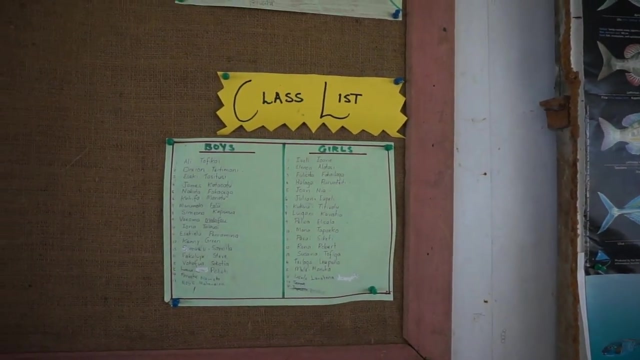 the kids are taught in English And all the kids here speak English very, very well. Here is the board organization board The different teams. Here is the class list- Boys and girls. Look at it, And I was correct. There is 30 kids here. 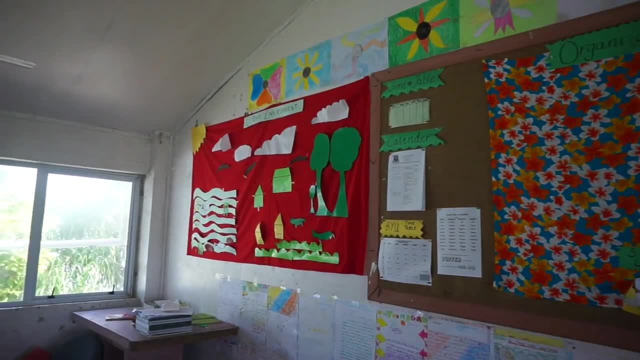 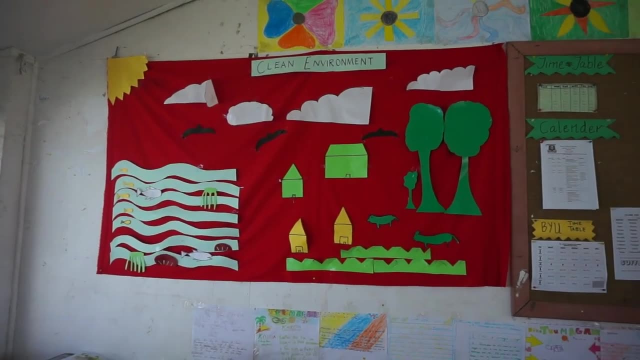 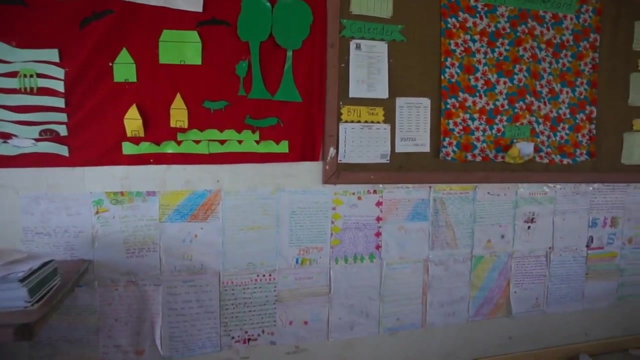 15 boys, 15 girls, Clean environment, Teaching them how to keep Tuvalu clean, And I must admit they are doing a relatively good job keeping the country clean compared to other countries here in the Pacific, And here is a different classroom. 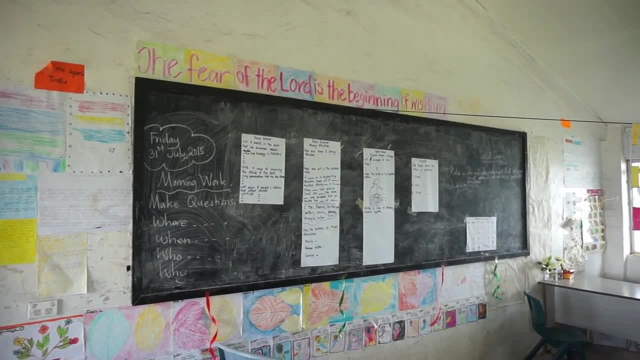 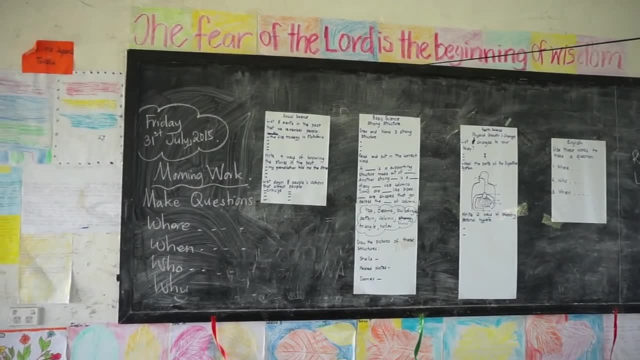 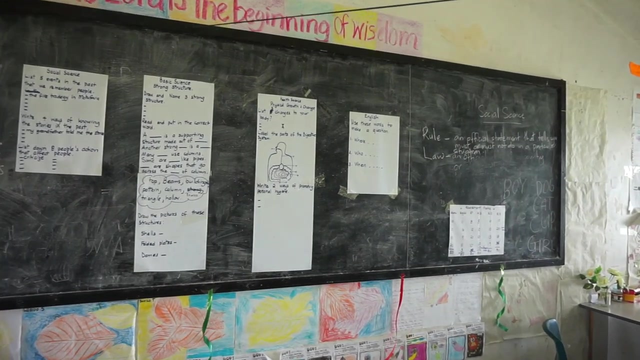 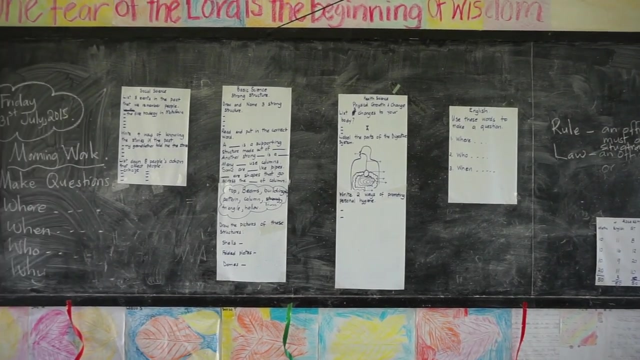 And it says: Fear of the Lord is the beginning of wisdom. That's the saying on top of the board, over the board right there, And you can see here the kids are learning English, health science, social science, basic science. 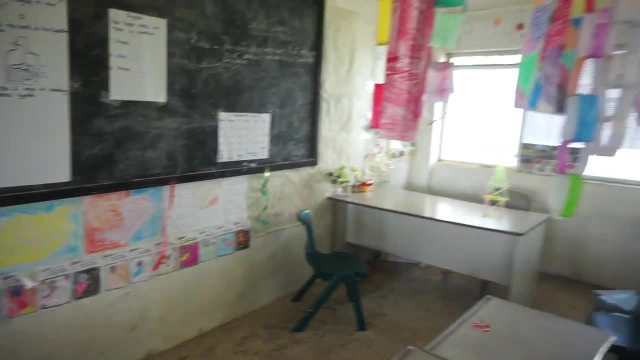 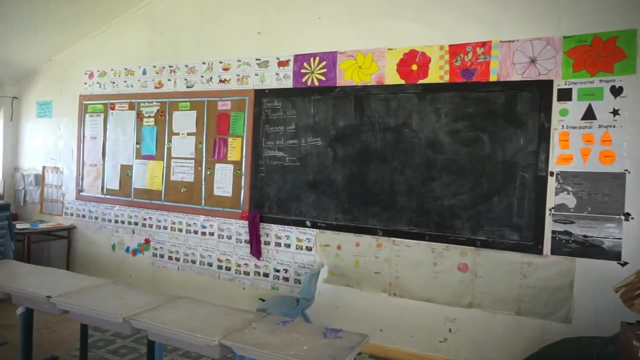 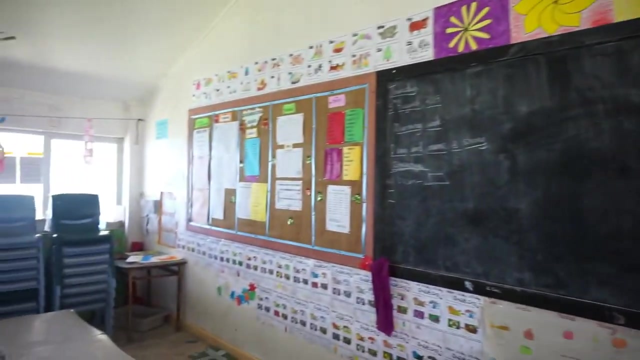 But they all are studying English now much better And it looks like they're taking teaching courses overzealous, And also they're doing so well with this plan, because each of these classes has a" And that's that. And then here: 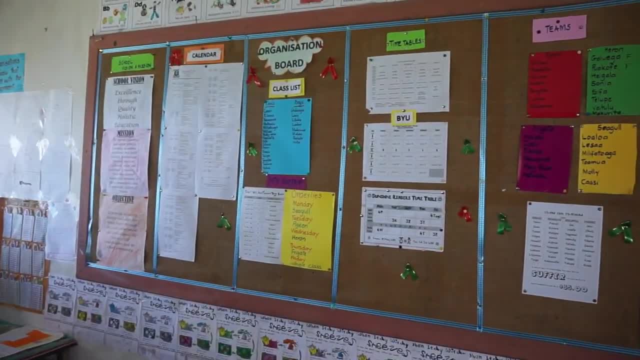 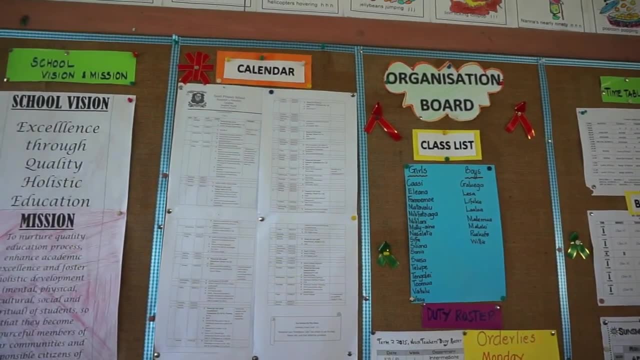 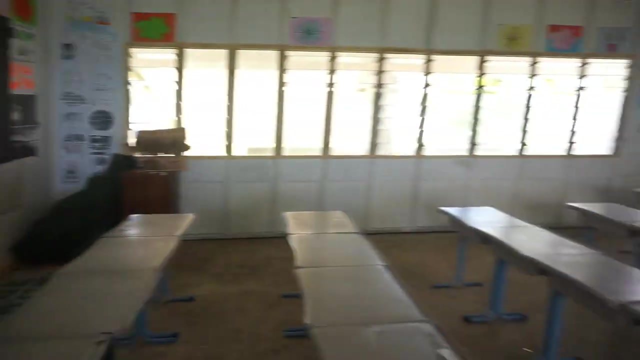 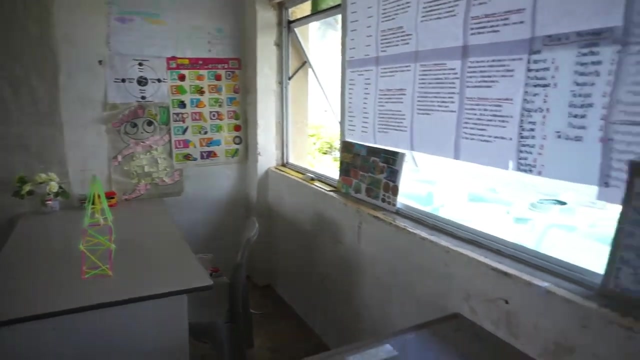 it says: powinna ser una escuela. Don't break it, Juegue. This is the job. Here is the general view and here is the teacher's desk. Here's a beautiful view, by the way of the lagoon. 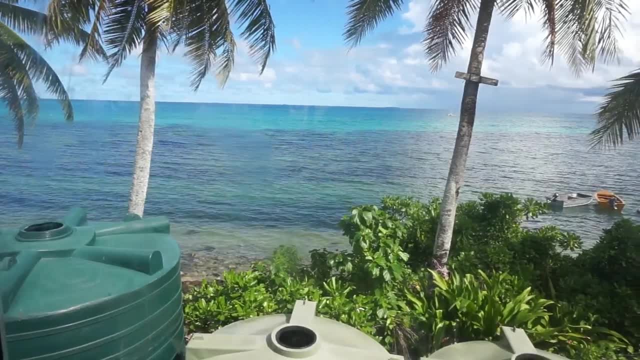 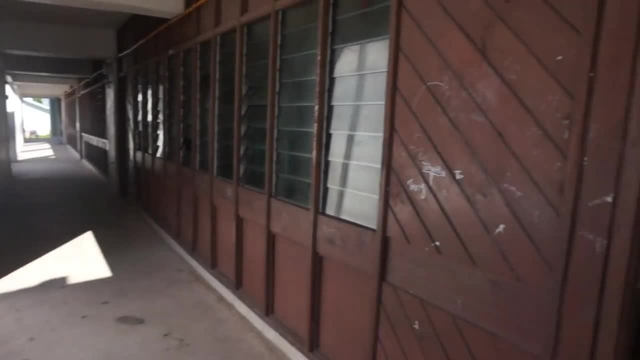 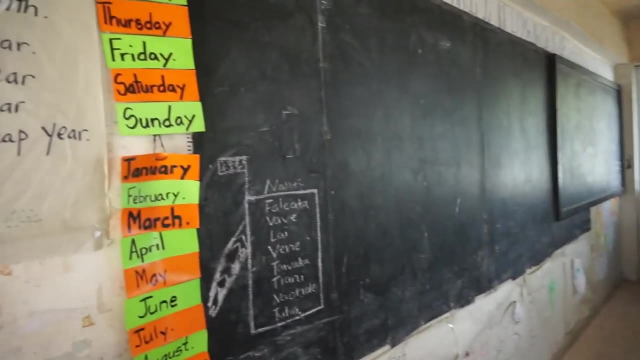 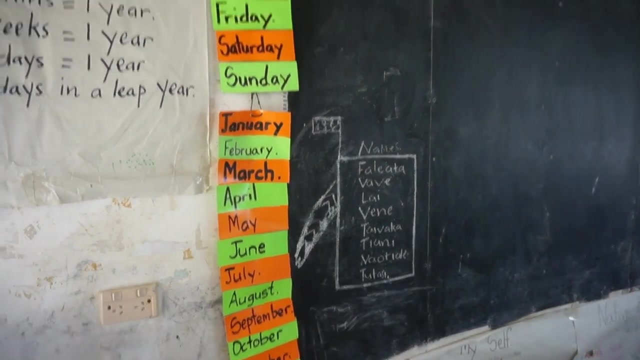 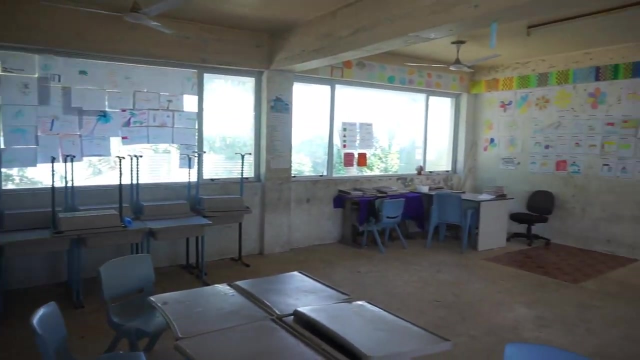 You can see the beautiful blue water. I am now downstairs, so let's visit one of the classrooms here You can see everything is in English. Here are the months and the days of the week: the alphabet. Every classroom is in English. 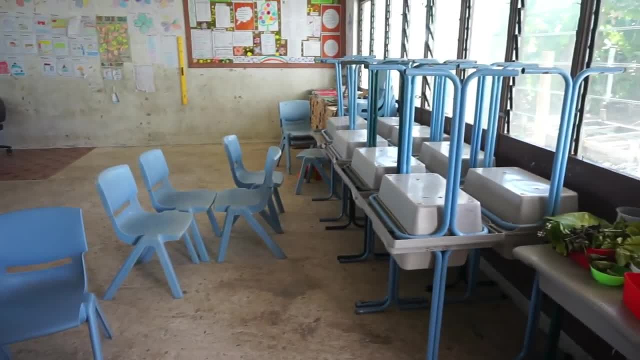 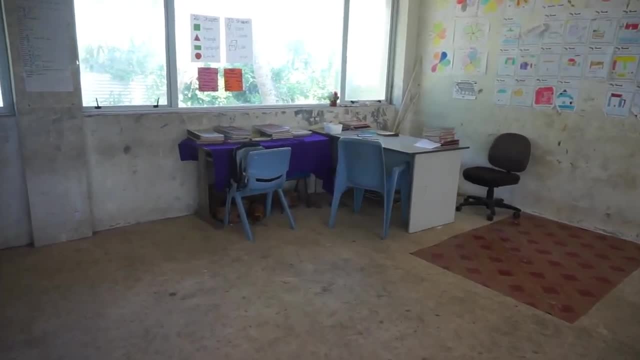 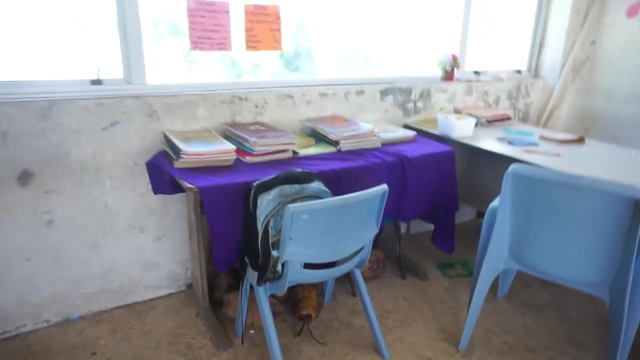 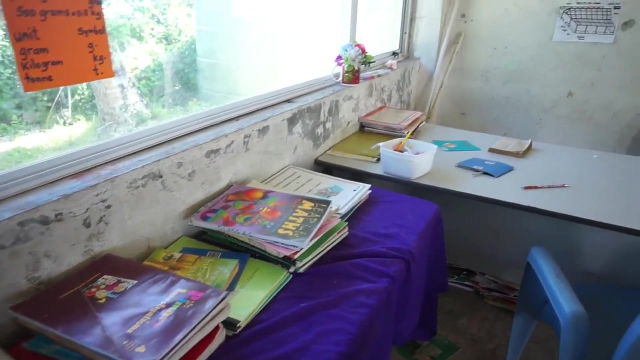 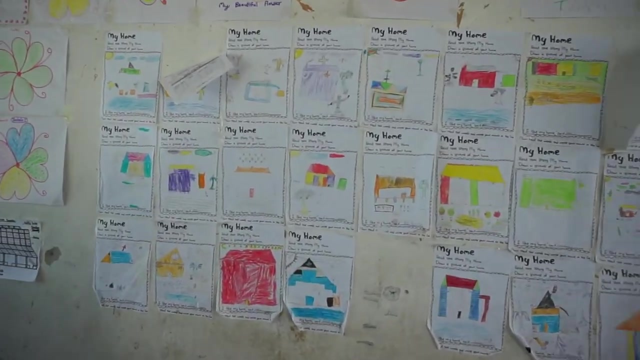 Same desks and chairs. One desk and one chair per student. Here is the desk of the teacher here. I am not sure what the coconuts under the desk are doing there. Right there, Books: Here is something interesting. Every kid here. 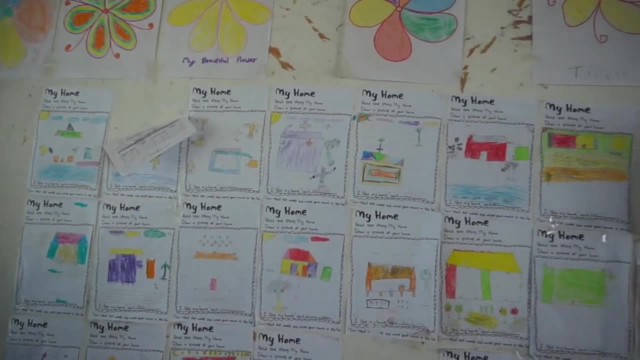 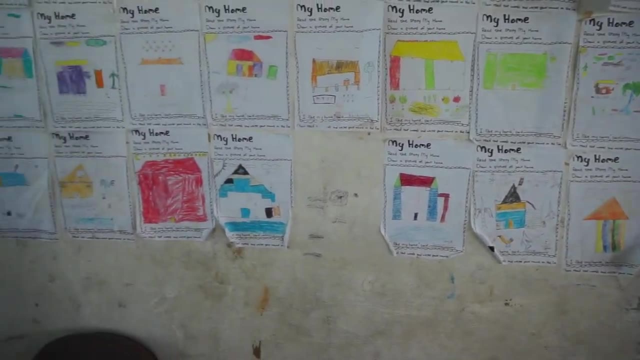 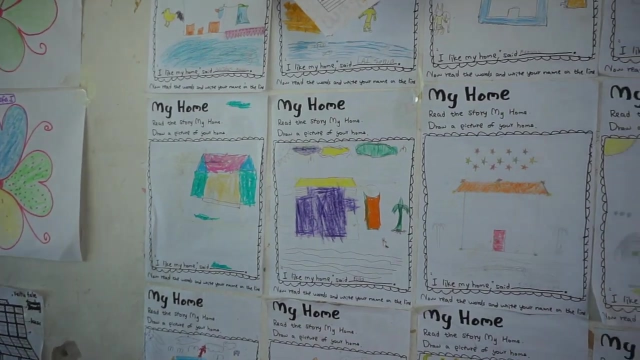 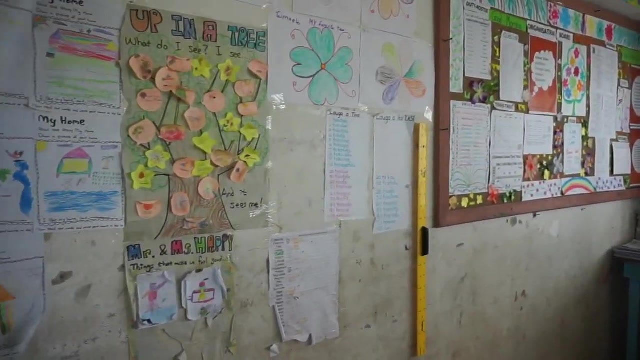 Every student here has drawn his home or her home. Look at this So you can see how kids here picture and imagine their homes. So this is certainly a classroom of very young kids, Probably about six or seven years old. I don't know what they're doing. 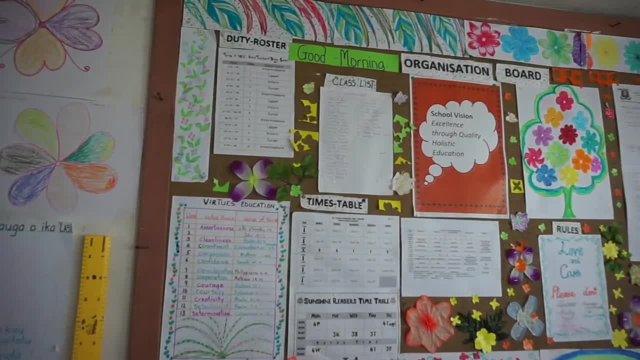 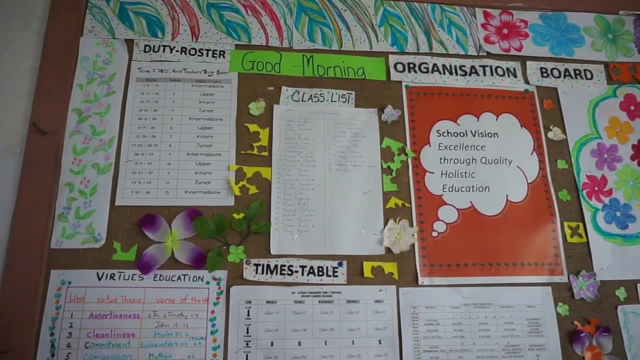 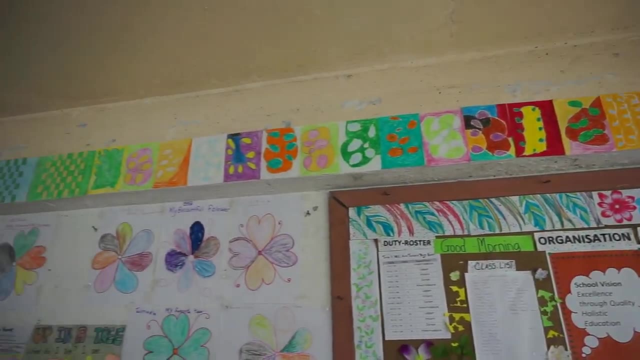 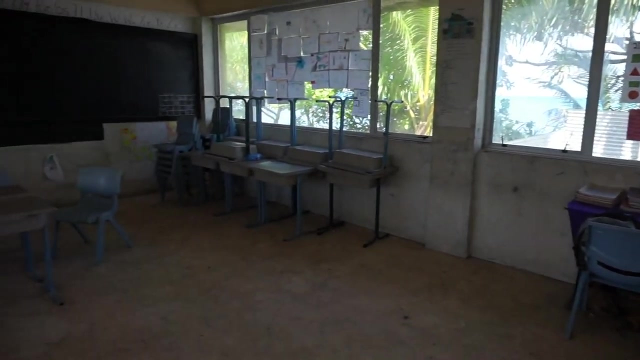 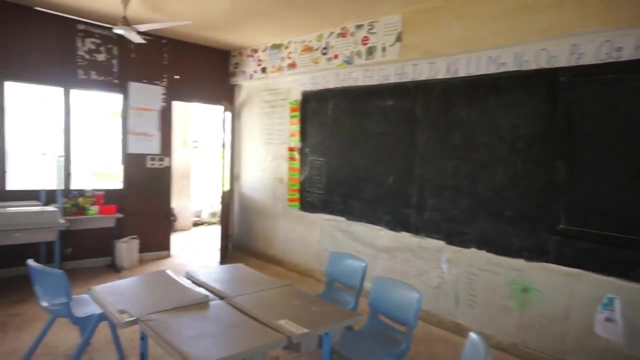 Okay. so now let's go up here. Yes, old, he has a class list with the boys and girls: 11 girls and 34 boys. lucky girls, look at this. yeah, these are definitely youngsters here. here's the overall look and feel of the classroom. now let's look at the books here, let's. 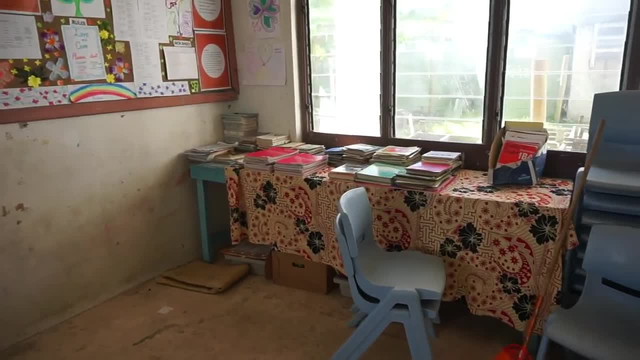 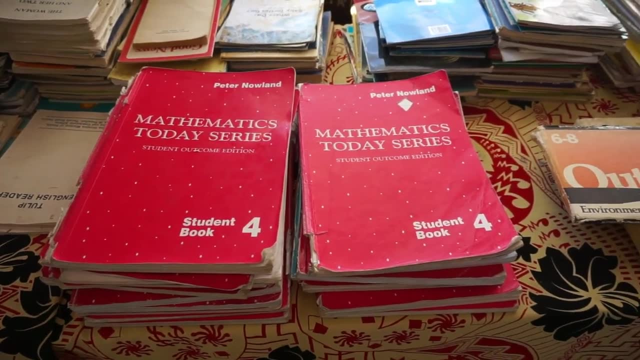 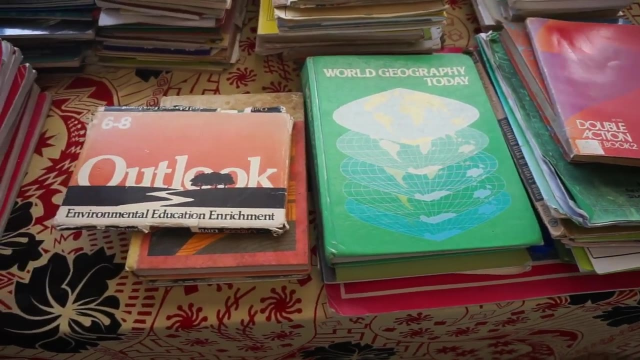 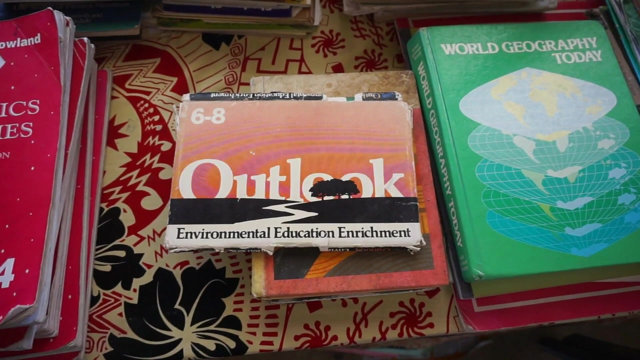 go to the books and see what do they teach them. here's a couple of books about mathematics, geography- the green one- and I'm surprised here- pleasantly surprised- that there is emphasis on the environment. we did see upstairs in one of the classrooms, emphasis about the environment. and here's a book says: 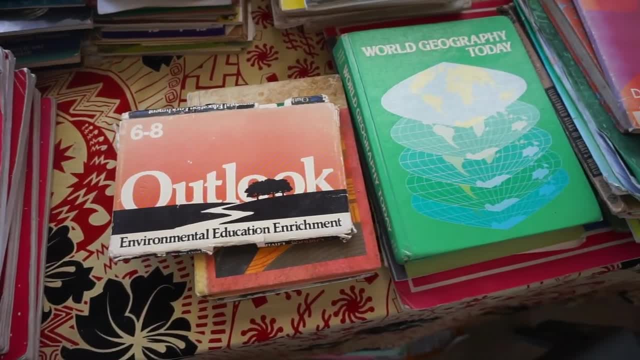 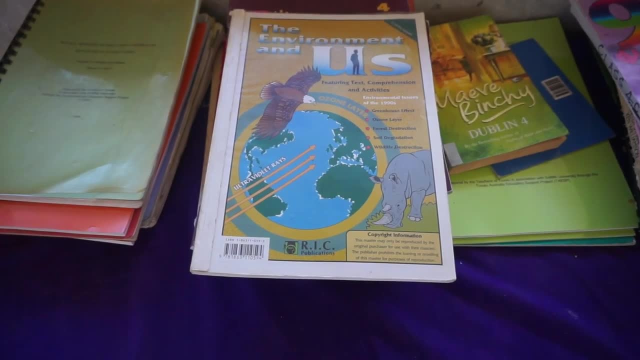 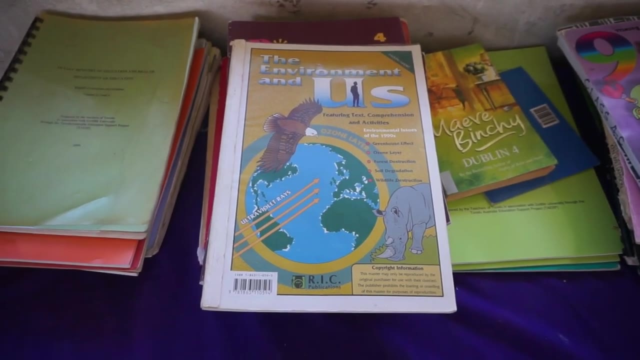 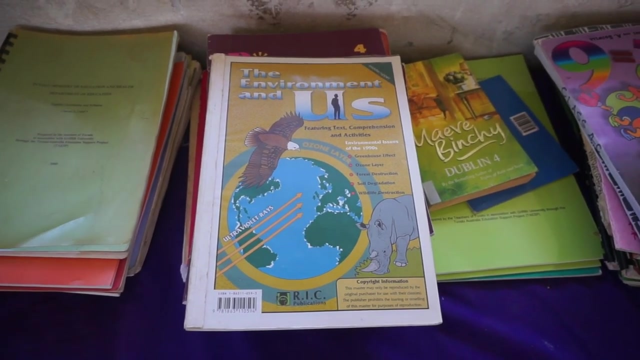 environmental education, enrichment. and I'm still in the same classroom. here's another book that says the environment and us. so they must teach their kids here from very young age how to take care of the environment, and Davalo really has no choice. it is such a small country, was so limited space if they don't take care of. 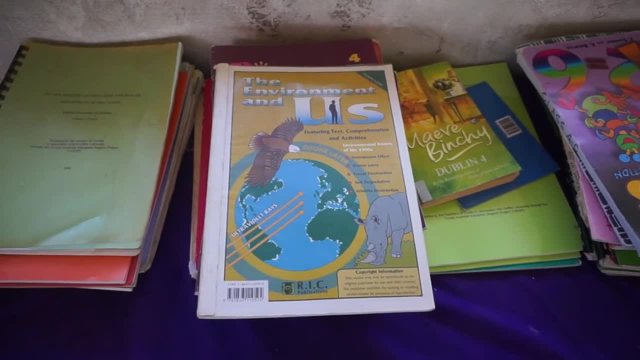 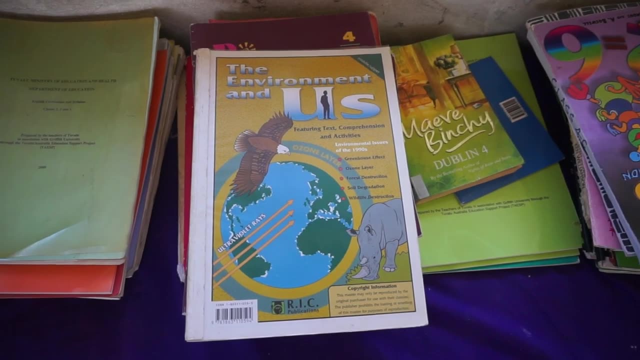 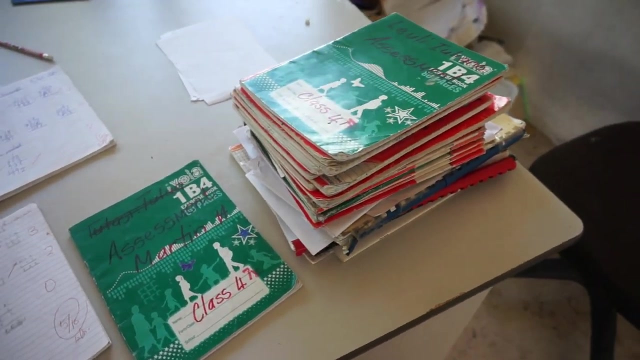 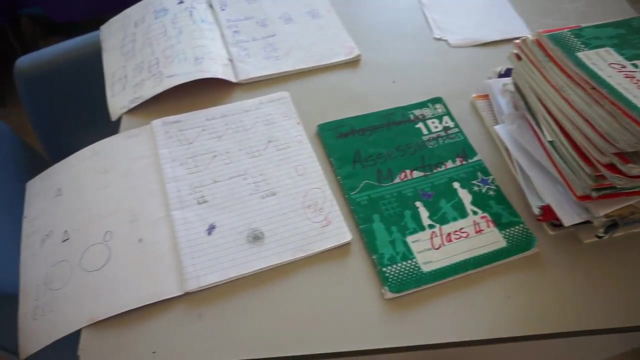 the environment. all country will be swimming in garbage. so I'm very, very pleasantly surprised here now. this stack of notebooks that you see here are quite obviously from the students here in university, if you are, if you finish here classroom, and let's look at a couple of them. you can see this is math and in 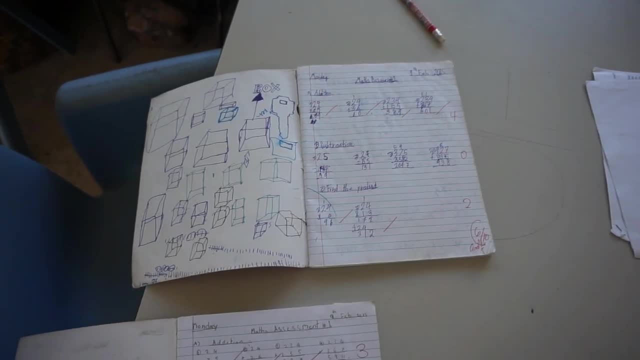 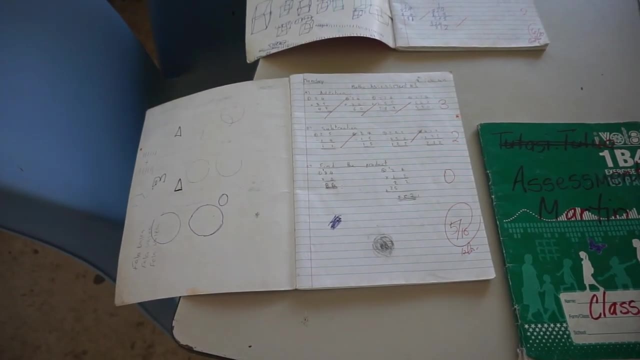 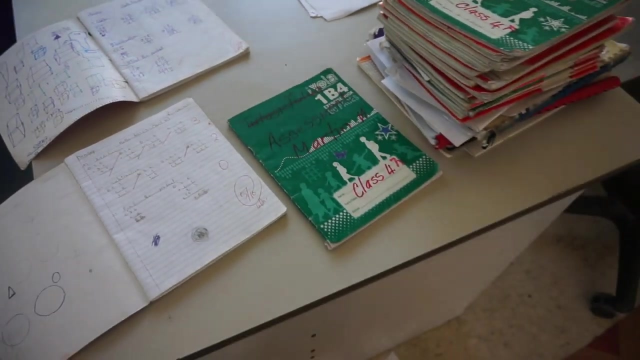 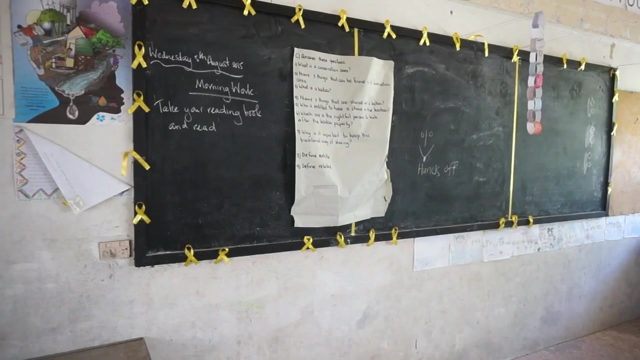 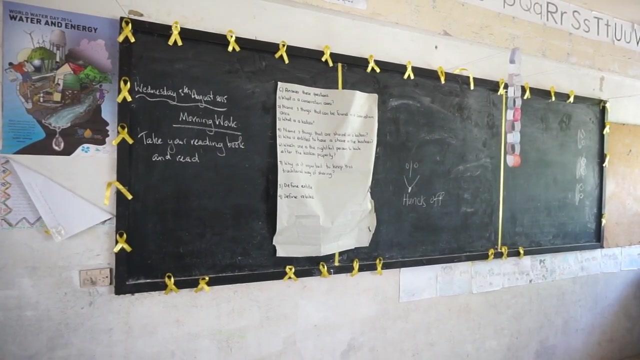 this particular case. the student here got six points out of ten and this student here got five points out of ten. you can see the red markings on the lower right corner. here's the view of the teachers desk and here's the last classroom we're going to look at and there is not going to show you this one. 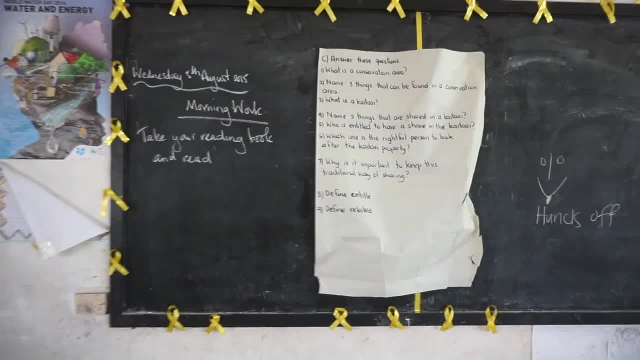 it's because of what's written here on the board. I want to go back to the theme of the class and I'm going to go back to the theme of the class and I'm going to go back to the theme of the class and I'm going to go back to the theme of the class and I brought up your attention about the. 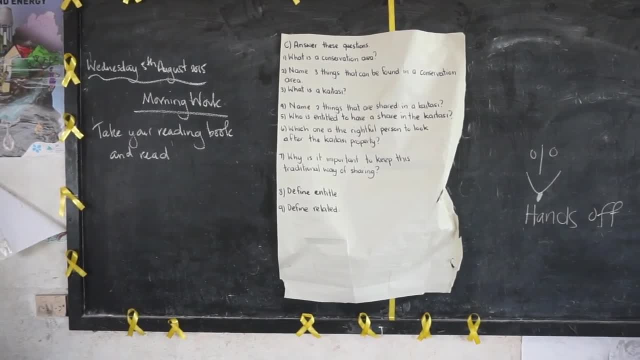 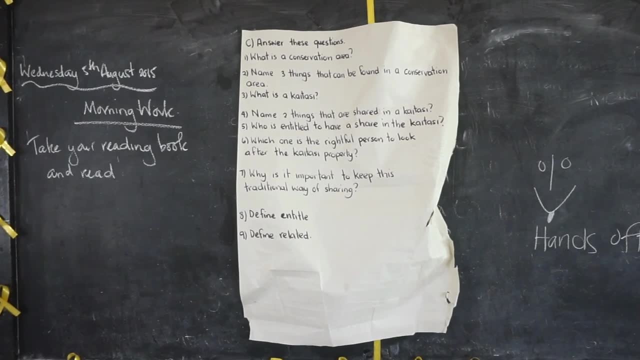 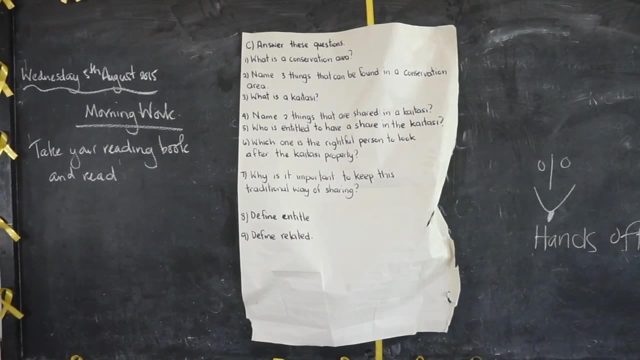 that I brought up your attention about the environment and here, on this piece of paper taped to the wall, to the board, it says: what is a conservation area? that's the number one question, and number two is name three things that can be found in a conservation area. the theme here is constantly the. 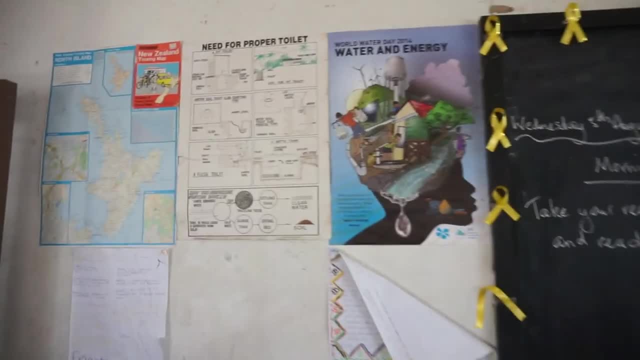 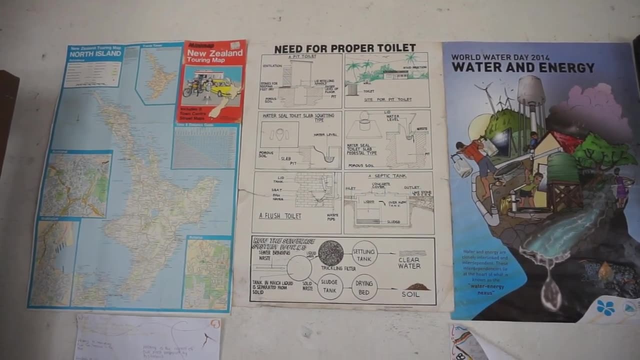 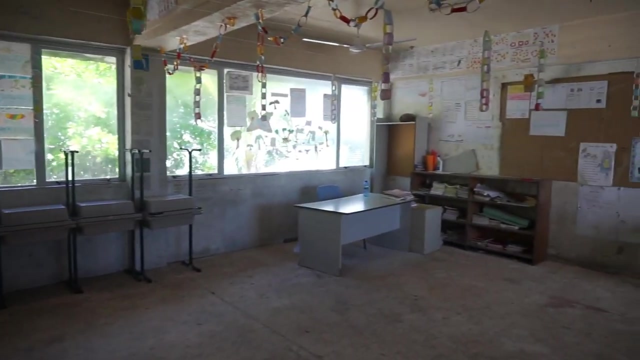 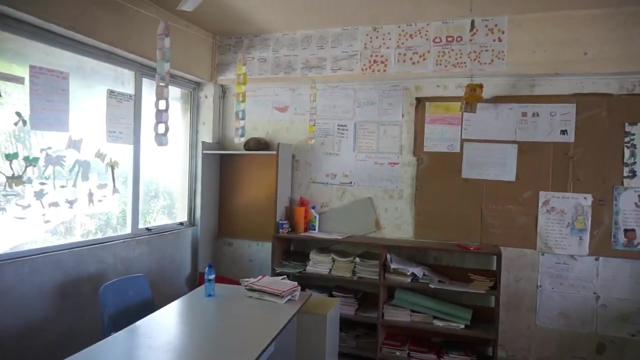 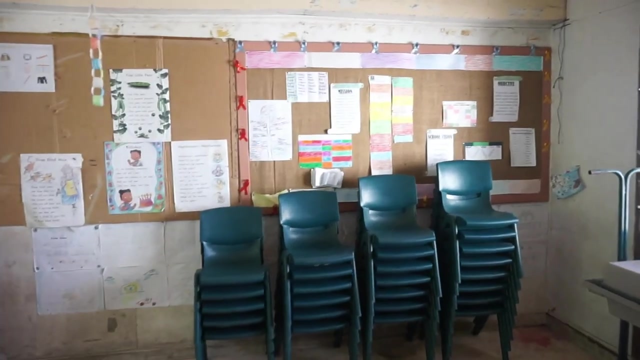 environment. look at this here: water and and environment. look at this here: water and and energy. the need for proper toilet. how do you have a proper toilet constructed? you can see these signs over there. so the overall theme, recurring theme in this classrooms is the environment. of course there are other themes here, but every classroom seems to have a. 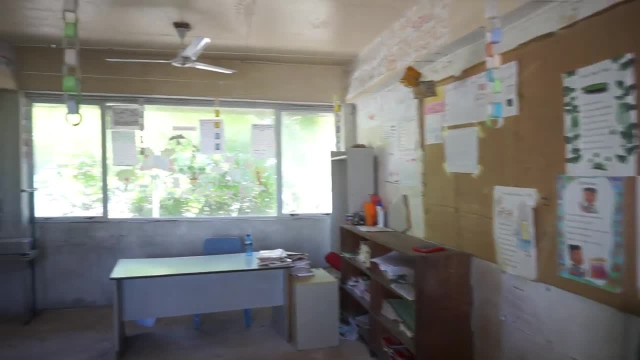 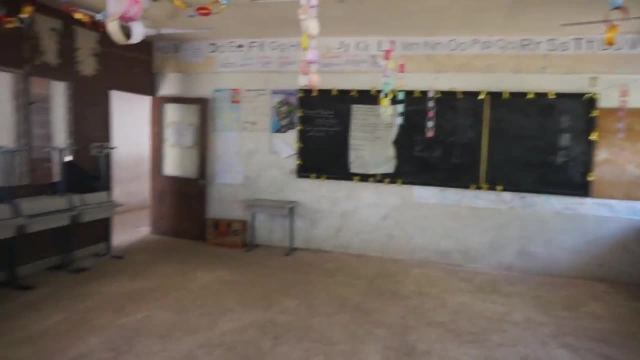 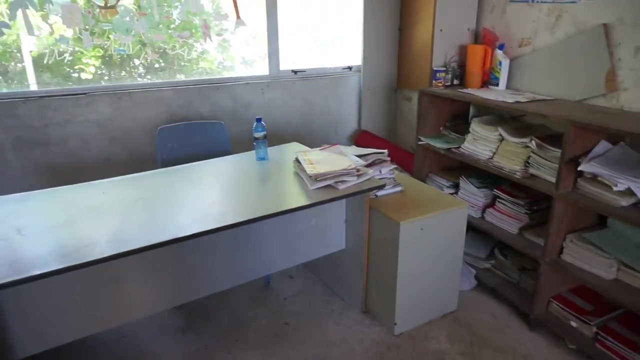 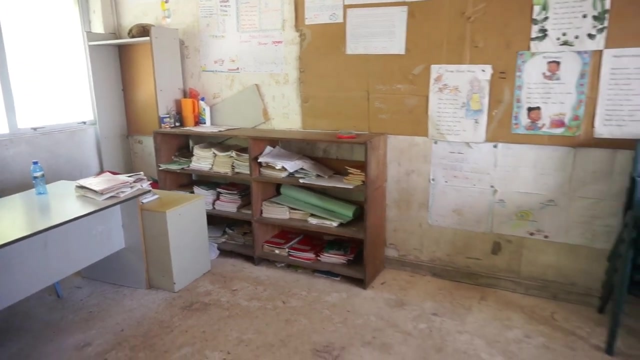 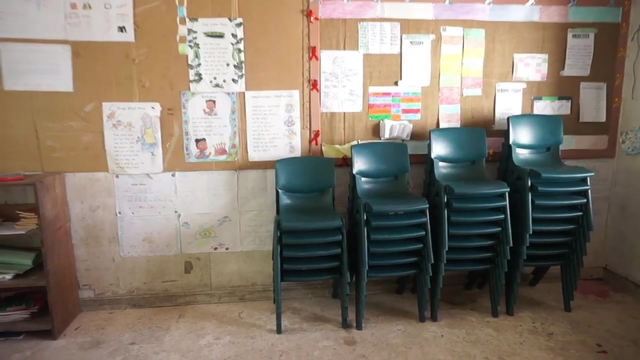 certain emphasis in the environment as well. you can see the decorations in this classroom, by the way, and same desks and chairs and, if you have the lagoon right there, the teachers desk note books. well, I hope you have enjoyed this tour. it's very unique tour of a primary school in Tuvalu in the Central Pacific, I doubt.